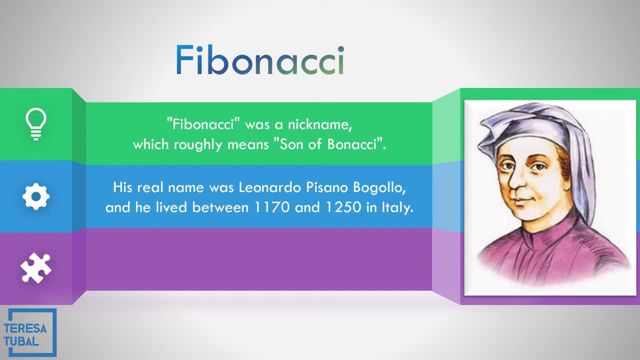 His real name was Leonardo Pesano Bugoglio and he lived between 1170 and 1250 in Italy, And he also helped spread the use of Hindu system. So the Hindu system is 0,, 1,, 2,, 3,, 4,, 5 and so on. 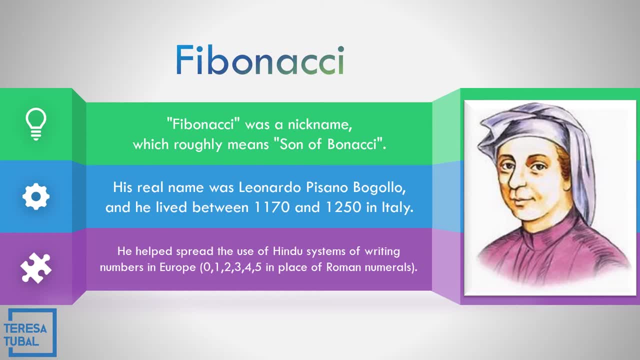 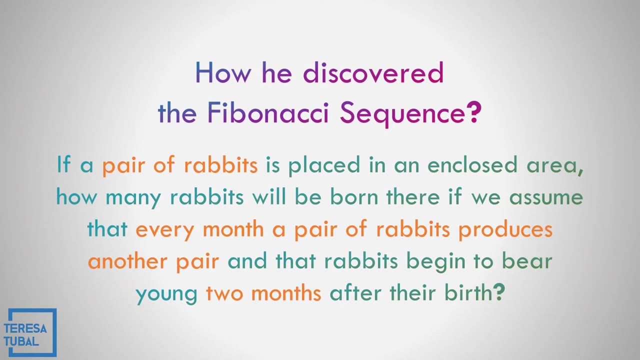 in place of the Roman numerals. As you remember, the Roman numerals is I, X, L, C, That is, the Roman numerals. How we discover the Fibonacci sequence? If a pair of rabbits is placed in an enclosed area, how many rabbits will be born there? If we assume that every month, a pair of rabbits produces? 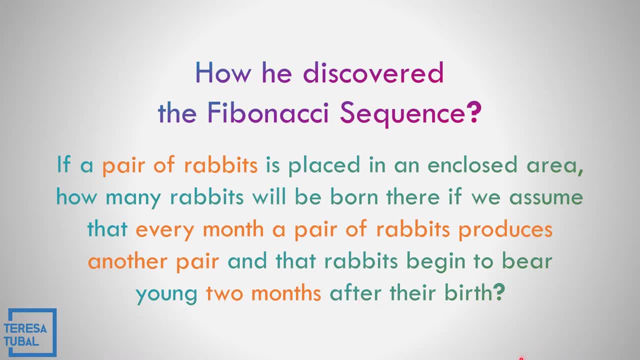 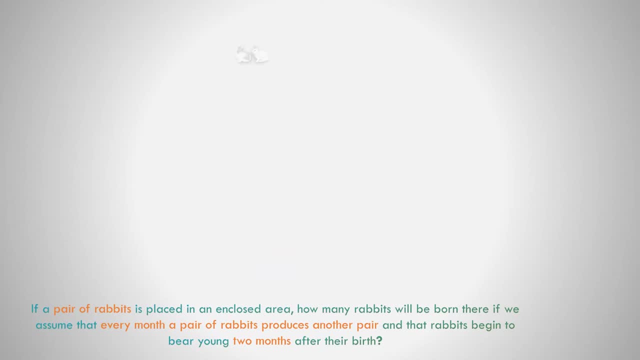 another pair and that rabbits begin to bear young two months after their birth. So let us see how Fibonacci sequence is discovered by observing the rabbits At the start. no rabbits are born as the initial pair have not time to be pregnant and born In the first month. one pair of rabbits is born In the second month. another one pair of rabbits is born. 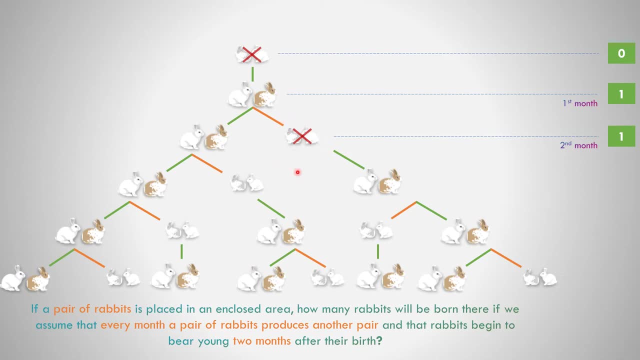 and the other one is born. So the first pair of rabbits is born and the other one is born. The other pair are not yet mature to bear young. In the third month, two pair of rabbits are born, while the other pair are not yet mature to bear young. In the fourth month, three pairs of rabbits. 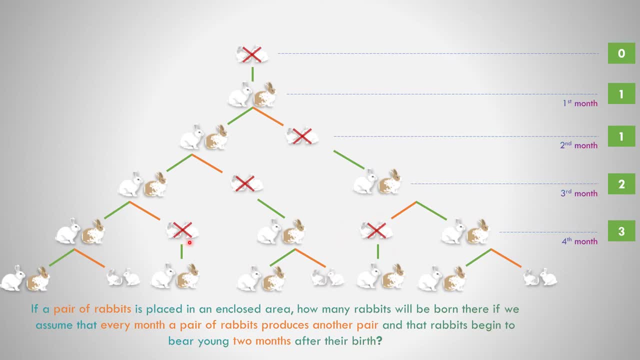 are born and the two pairs are not yet mature to bear young. In the fifth month, five pairs of rabbits are born and three rabbits are not yet mature to bear young. So, as you can see in Fibonacci sequence, the Fibonacci sequence is not yet mature to bear young. So as you can see in Fibonacci sequence, 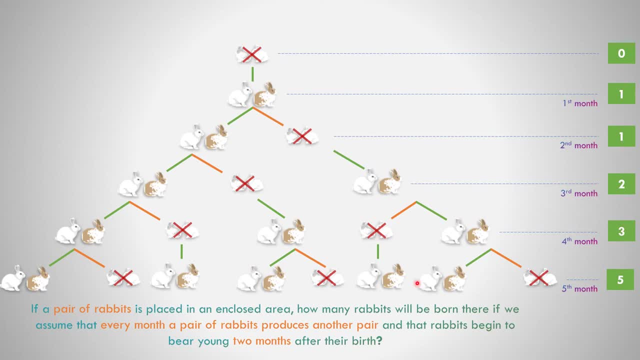 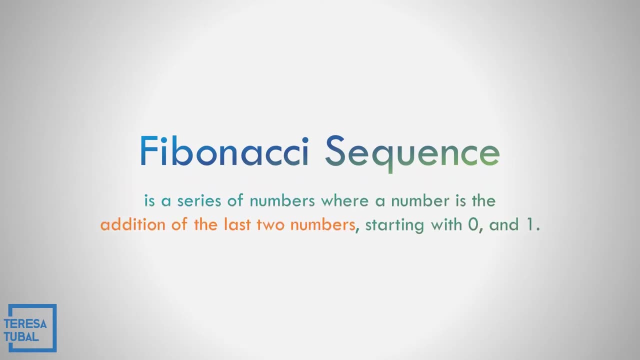 the Fibonacci sequence is not yet mature to bear young. So, as you can see, in Fibonacci sequence it is always 0,, 1,, 1,, 2,, 3, and 5.. Fibonacci sequence is a series of numbers that, were a number is the addition of the last two. 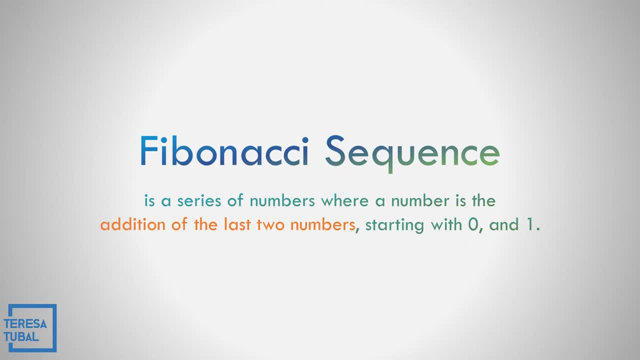 numbers starting with 0 and 1.. So the Fibonacci sequence rule: F sub n is equal to F sub n minus 1, plus F sub n minus 2, where F sub n is equal to F sub n minus 1 plus F sub n minus 2, where F sub n is equal to F sub n minus 1 plus F sub n minus 2,. 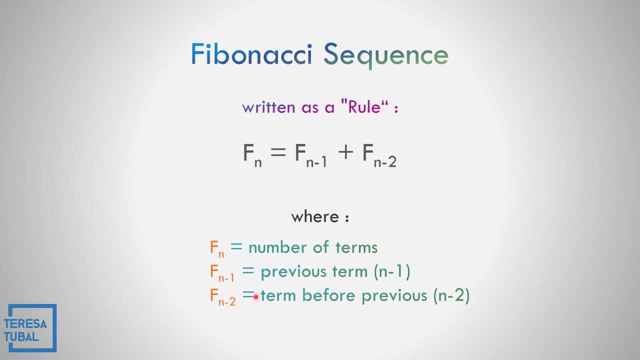 and F sub n minus 1 is the number of term and F sub n minus 1 is the previous term, and the F sub n minus 2 is the term before the previous. F sub n minus 2 is the 2004.. 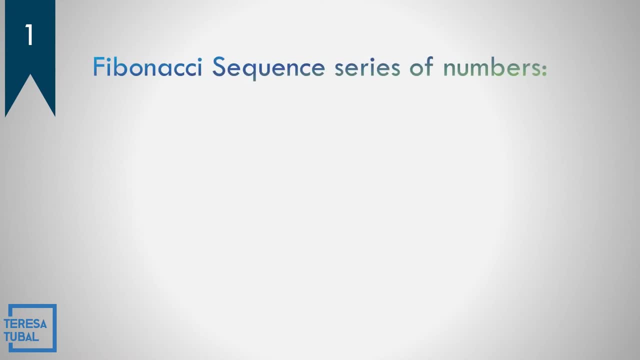 Fibonacci sequence series of numbers are 0,, 1,, 1,, 2,, 3,, 5,, 8,, 13,, 21, and 34.. are 0,, 1,, 1,, 2,, 3,, 5,, 8,, 13,, 21, and 34.. 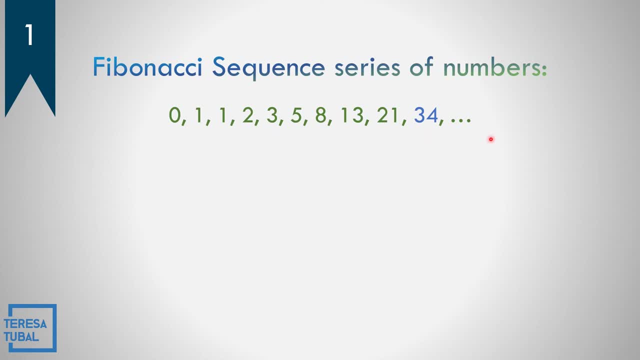 Are 0,, 1,, 1,, 2,, 3,, 5,, 8,, 13,, 21, and 34.. How to get those consecutive numbers? So, as you can see, we may add one last number. 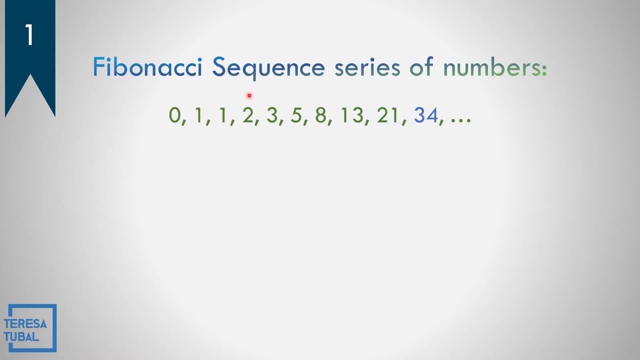 add: 1 plus 0 is 1, 1 plus 1 is 2, 2 plus 1 is 3, 3 plus 2 is 5, 5 plus 3 is 8, 8 plus 5 is 13, 13 plus. 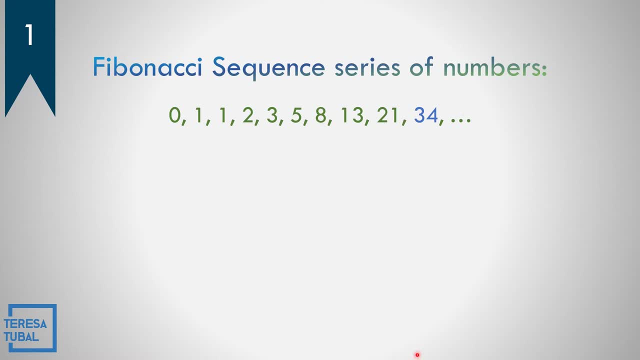 8 is 21. 21 plus 13 is 34. what do you think is the next number after 34? so the rule f sub n is equal to f sub n minus 1 plus f sub n minus 2, so that is f sub 11. if we count, this is 1, 2, 3, 4, 5, 6, 7, 8. 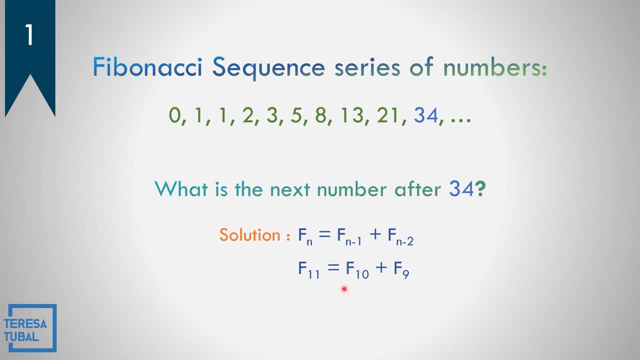 9, 10, 11. so the unknown is f sub 11 is equal to 11 minus 1, that is, f sub 10, 11 minus 2, 9, so f sub 9. so f sub 11 is equal to the previous. the unknown before the previous is 34 and before the previous: 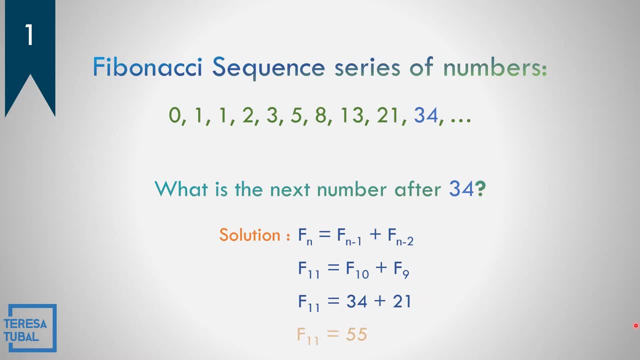 is 21. so 34 plus 21 f sub 11 is equal to 55. so it means the next number after 34 is 55. in the given Fibonacci sequence series of numbers, what is the next number after 55? so the formula or the rule f sub n is equal to f sub n minus 1 plus f sub n minus 2. so it means the unknown is 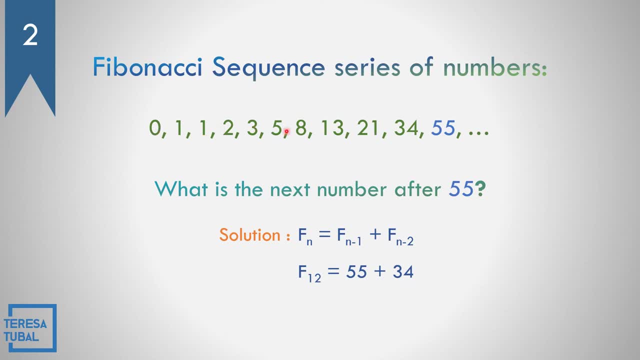 f sub 12. so if we count 1, 2, 3, 4, 5, 6, 7, 8, 9, 10, 11, 12, so f sub 12, so f sub n minus 1, that is the previous before the unknown. so that is 55 and that is the next number after 55. so the next number: 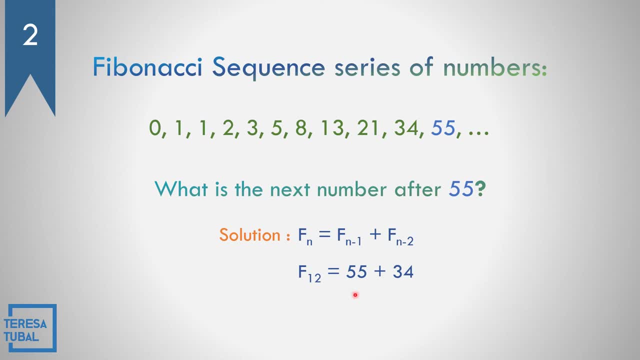 before the previous, that is 34. so 55 plus 34 the answer is equal to 89. so the next number after 55 is 89. question number three: what is the next number after 89? so again, the formula f sub n is equal to f sub n minus 1 plus f sub n minus 2. so the unknown now is the 13th. so if we 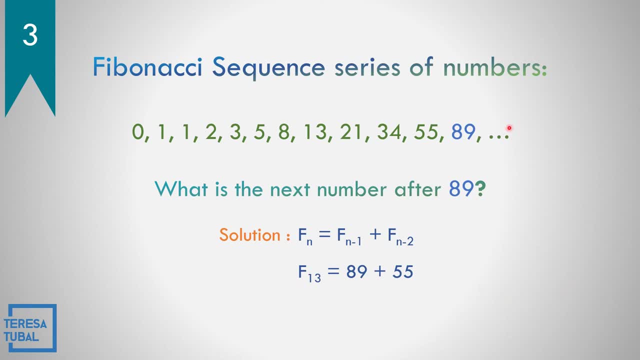 get the value of the f sub 13. the previous before the unknown is 89 and then the term before the previous is 55. so 89 plus 55 the answer is equal to 144. so the next number after 89 is 144 in the given 13, 21, 34 and 55. what do you think is the next two terms? so the rule? 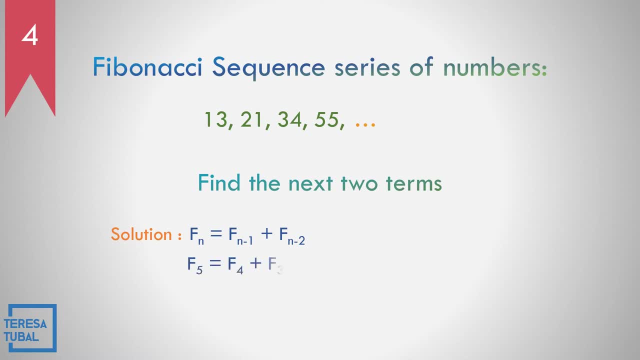 f sub n is equal to f sub n minus 1 plus f sub n minus 2. so the unknown is the fifth term. so the fifth term is equal to f sub 4 is. this is the previous and the term before the previous is 34, so that becomes: 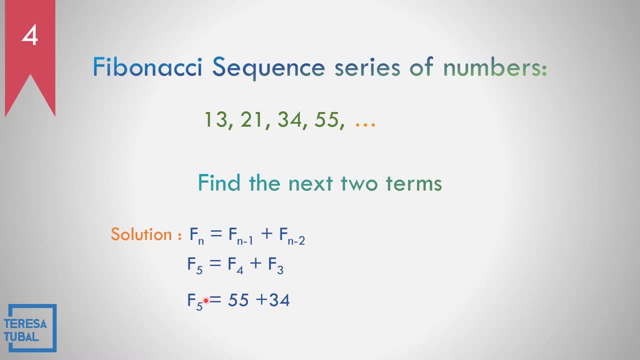 f sub 5 is equal to 55 plus 34. so 55 plus 34 f sub 5 is equal to 89. how about the next after 89? so that is f sub 6. f sub 6 is equal to the previous previous f. 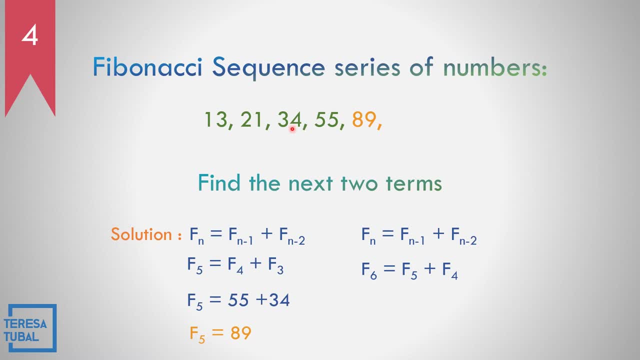 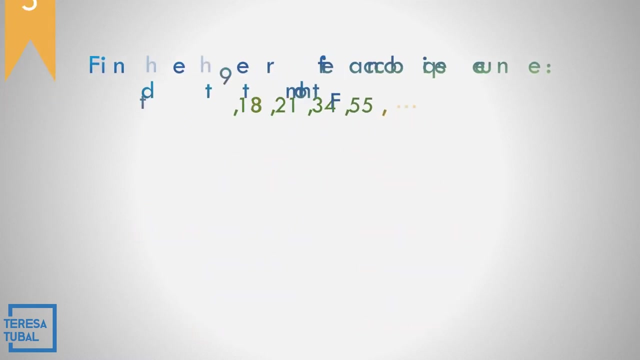 sub 5 and the term before the previous is f sub 4. so that is f sub 6 is equal to 89 plus 55. so 89 plus 55, the answer is equal to 144. find the ninth term of the Fibonacci sequence: 8, 13, 21, 34 and 55. so, as you can see, the first term is: 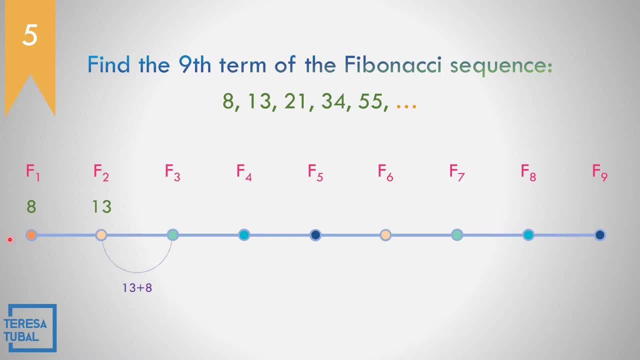 eight, the second term 13. the third term is 13 plus 8. it is 21, 21 plus 13, the answer is 34, 34 plus 21, it is 55, so 55 plus 34. f sub 6 is 89, so 89 plus 55. f sub 7 is 144, so 144. 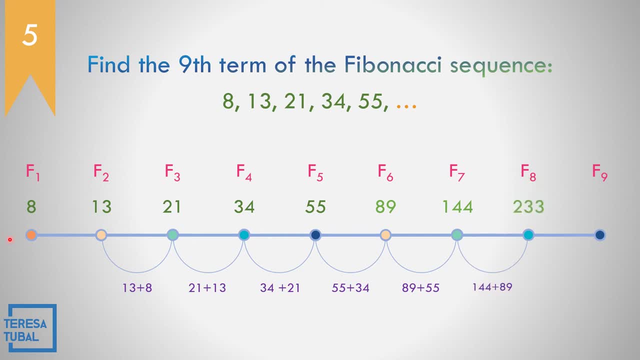 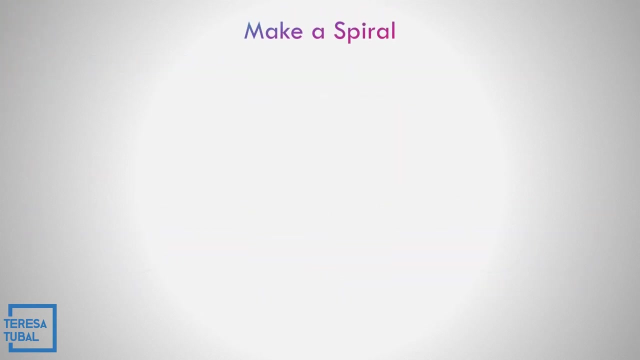 plus 8, F sub 8 is 233, and then 233 plus 144, so the F sub 9 is equal to 377.. So the ninth term of this given Fibonacci sequence, the answer is equal to 377.. So let us see in the diagram the example of Fibonacci sequence. 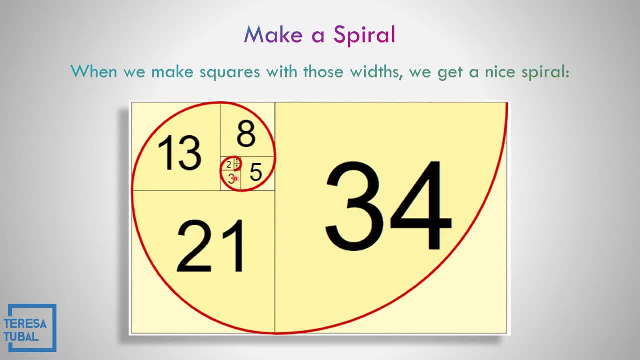 So 1 plus 1,, 2,, 2 plus 1,, 3,, 3 plus 2, 5,, 5 plus 3, 8,, 8 plus 5,, 13,, 13 plus 8,, 21,, 21 plus 13 is 34.. 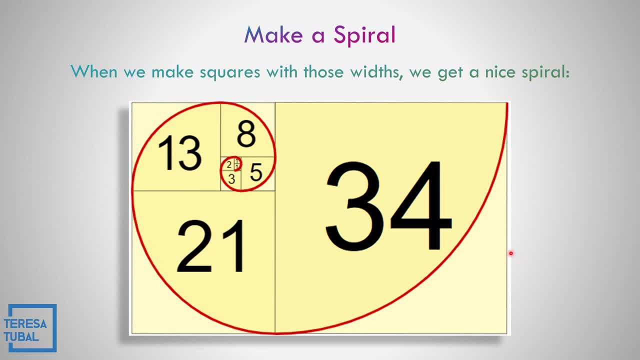 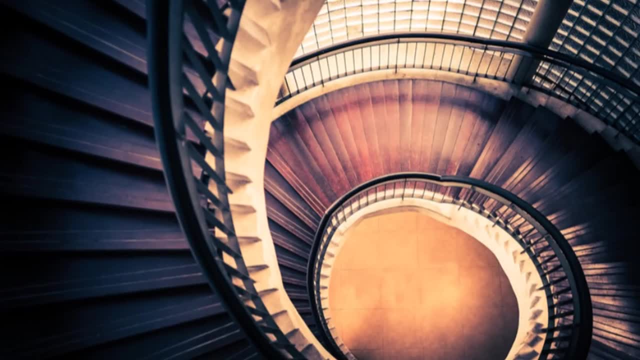 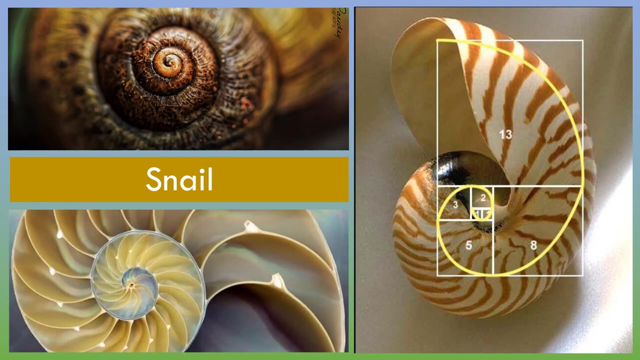 So when we make square with those widths we get a nice spiral. So these are the example of the spiral. Example of Fibonacci sequence: is this there So you can just pick it up, or you can see it on the screen? Other Fibonacci sequence that you will see in the nature like a snail. 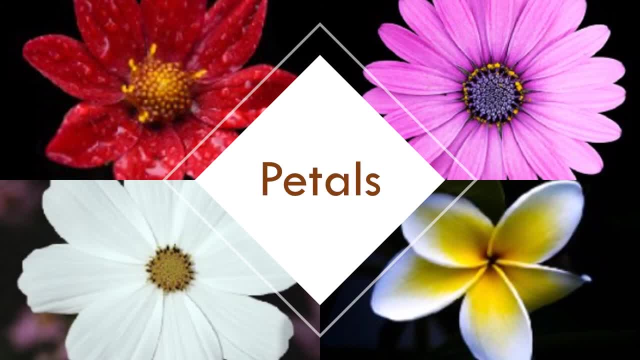 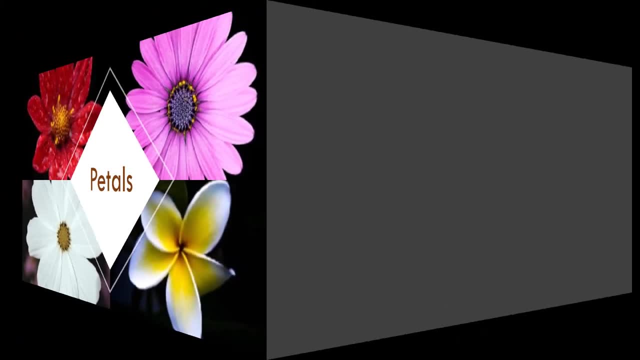 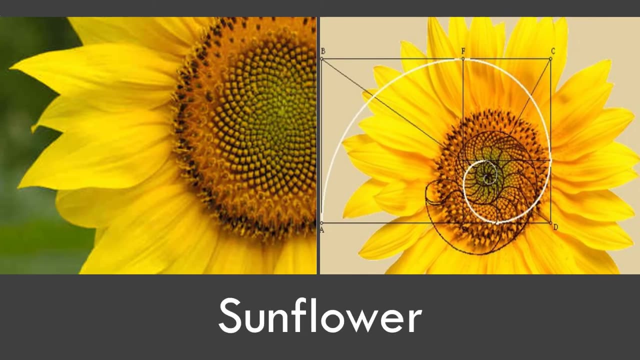 You can see also the Fibonacci sequence in the petals of the flowers. The petals of the flowers have 5,, 8, and so on. We can also see the Fibonacci sequence in the sunflower, As you can see at the center of the sunflower. 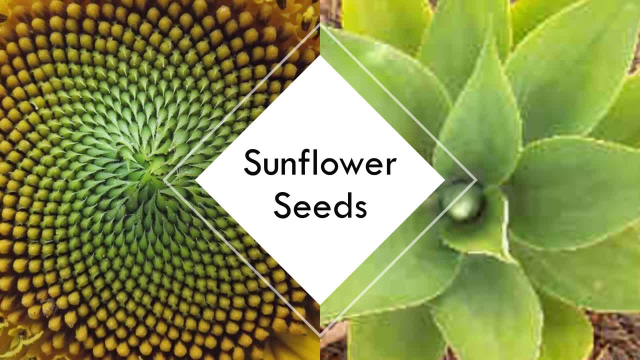 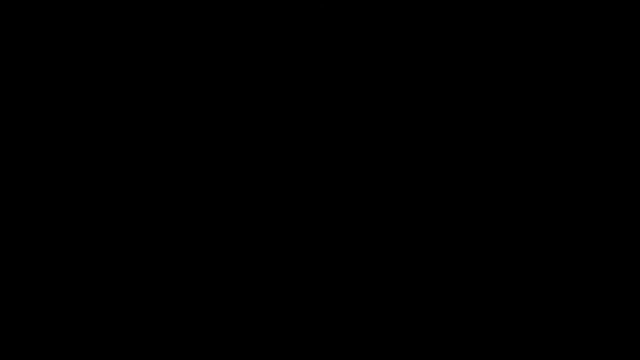 We can see also in the sunflower seeds. some examples that we can see: Fibonacci sequence. You can see the beauty of nature that have Fibonacci sequence. Fibonacci sequence is the beauty of nature. Fibonacci sequence is the beauty of nature. Fibonacci sequence is the beauty of nature.